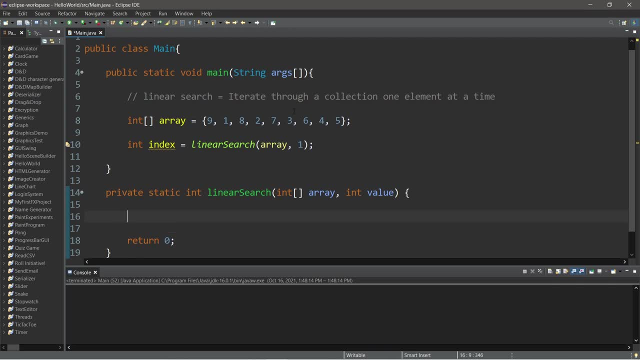 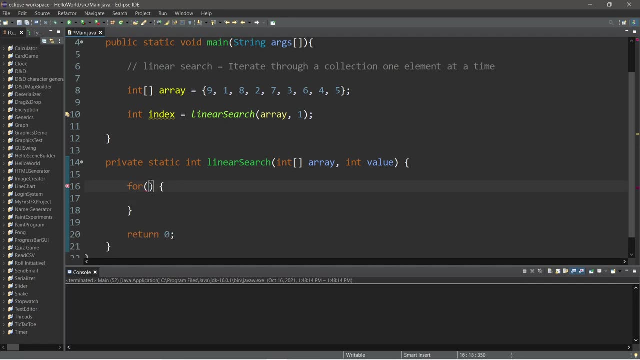 Ok, with a linear search, all we need to do is loop through our array one element at a time. So we can do that with the for loop. So let's set int i our index equal to 0.. We will continue this. as long as i is less than our array's length, that increment 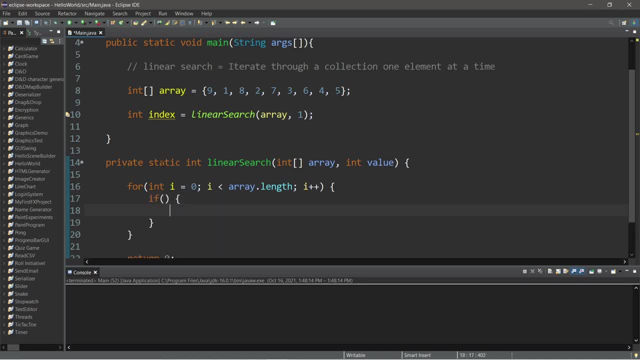 i by 1.. What we're checking with an if statement is to see if our array at index of i is less than our array's length, that increment i by 1.. What we're checking is to see if our is equal to the value that we're searching for this parameter. If it is, then let's return whatever. 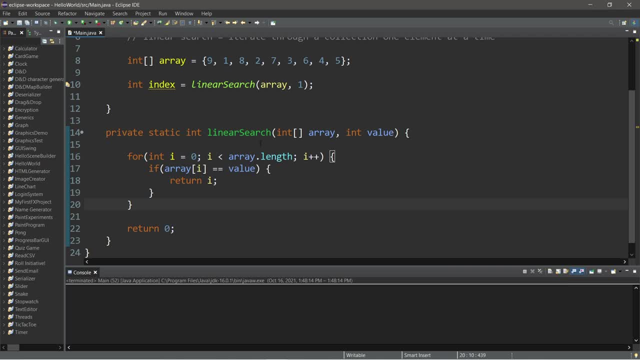 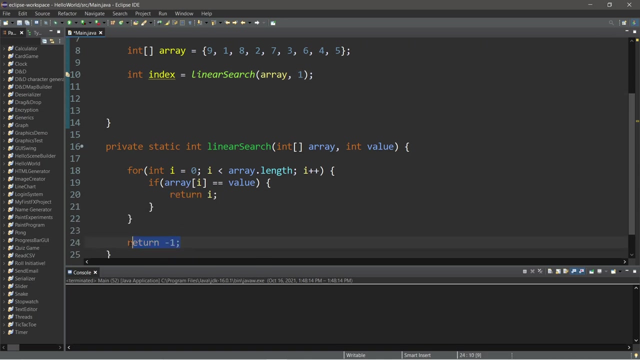 our index is i. If we do not find it after iterating through our entire array, let's return negative one as a sentinel value, and that's all there is to it, to our linear search function. So back within our main function, let's check to see if the value returned does not equal negative. 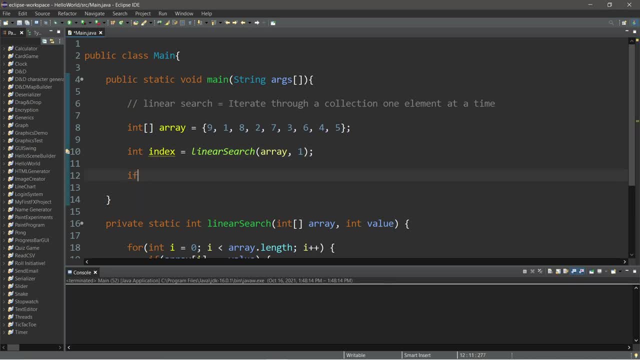 one, That means that we found our value. so with an if else statement, let's check to see if index does not equal negative one, That means that we have found our element. so let's print element found at index plus index. else let's print element not found: systemoutprintln element. 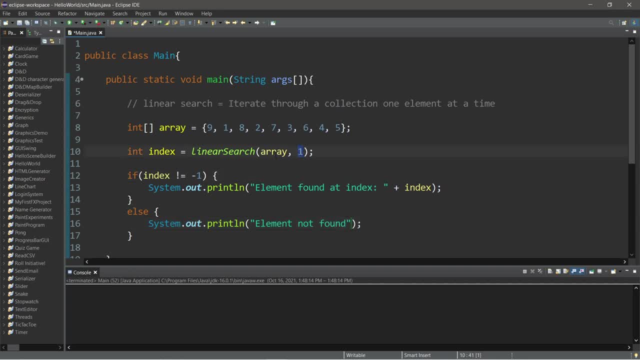 not found. So if we're searching for the value that we're searching for, let's return negative one. That means that we found our value, the number one. we would find that at index one, zero one. If we search for five, that is found at 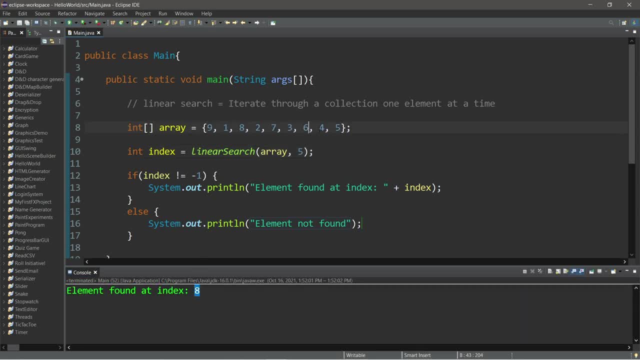 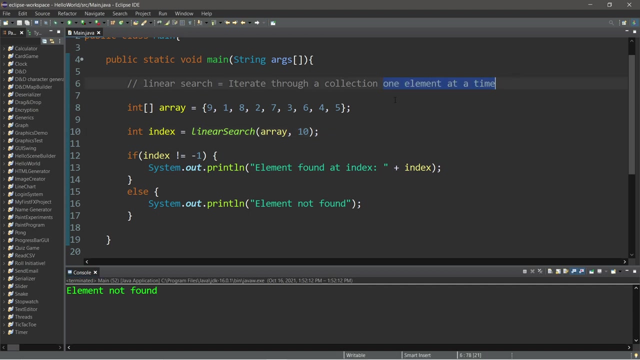 index: eight, zero, one, two, three, four, five, six, seven, eight. If there's some number that's not in here, like 10, then this will print element not found. So yeah, that's the idea behind a linear search. We iterate through some collection, one element at a time. It's slow for large data sets, but it's. 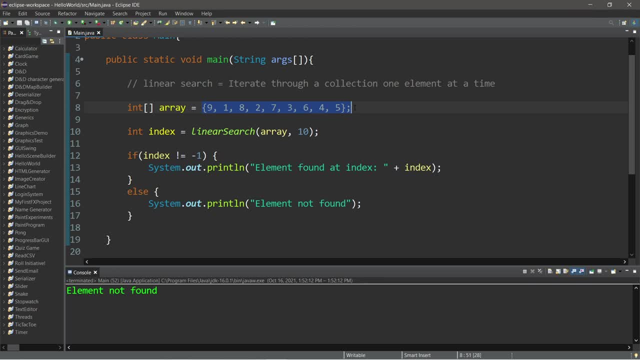 fast for small to medium data sets. This would be a small data set and they do not need to be sorted. That's a huge advantage. So yeah, everybody, that is a linear search. If you would like a copy of this code, I'll post this to. 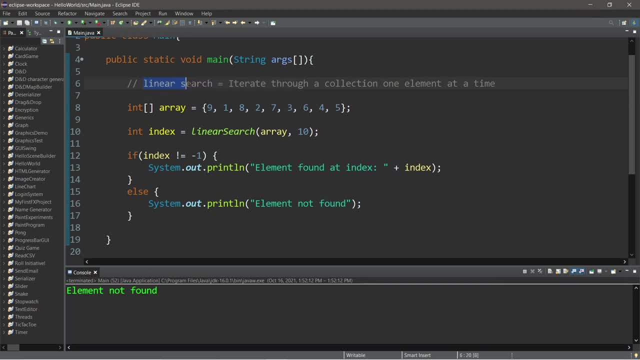 the comment section down below. And well, yeah, that is a basic linear search in computer science, I guess.